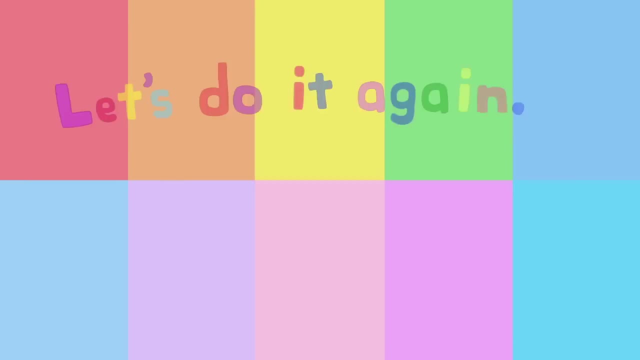 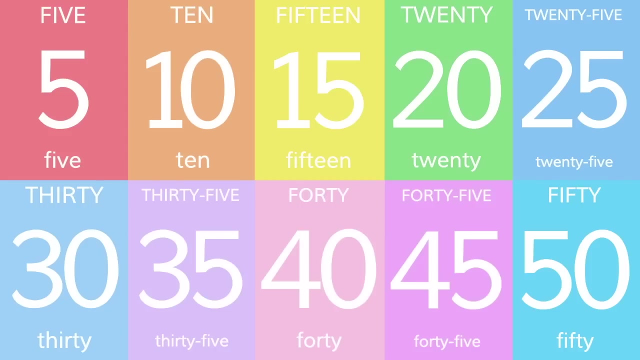 Let's do it again, but much more quickly, starting from zero: 5, 10,, 15,, 20,, 25,, 30,, 35,, 40,, 45,, 50.. 5, 10,, 15,, 20,, 25,, 30,, 35,, 40,, 45,, 50. 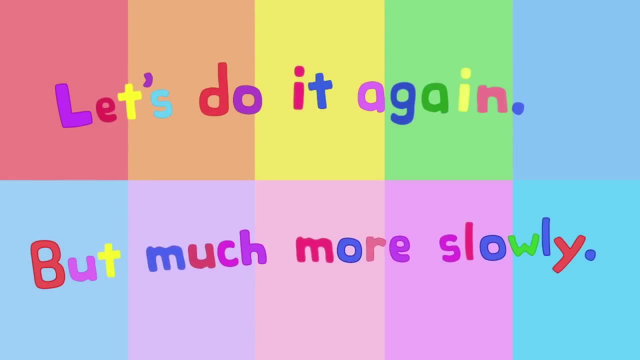 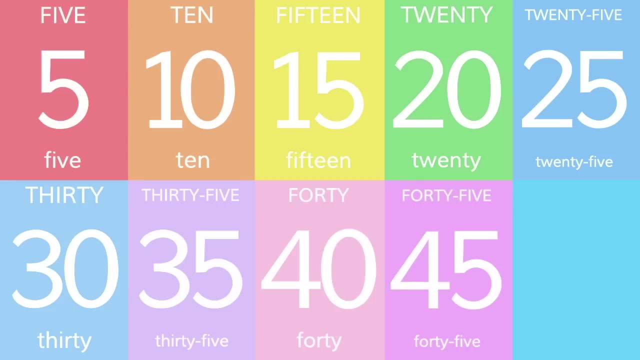 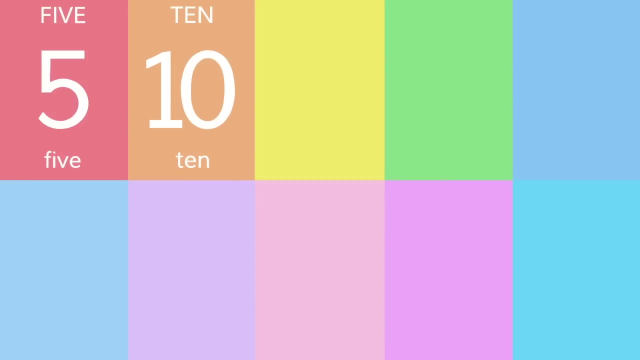 Let's do it again. 5,, 10,, 15,, 20,, 25,, 30,, 35,, 40,, 45,, 50.. 5,, 10,, 15,, 20,, 25,, 30,, 35,, 40,, 45,, 50. 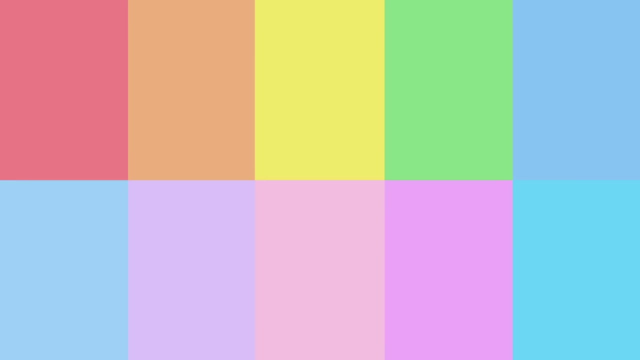 Counting by fives, I know you can do it up to 100, starting from zero: 5, 10, 15,, 20,, 25,, 30,, 35, 40, 45, 50, 55, 60,, 65,, 70,, 75,, 80,, 85,, 90,, 95. 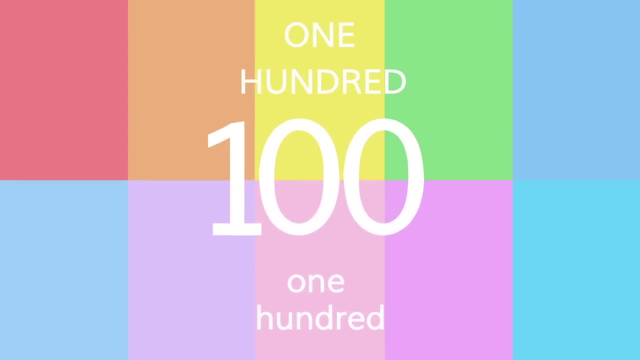 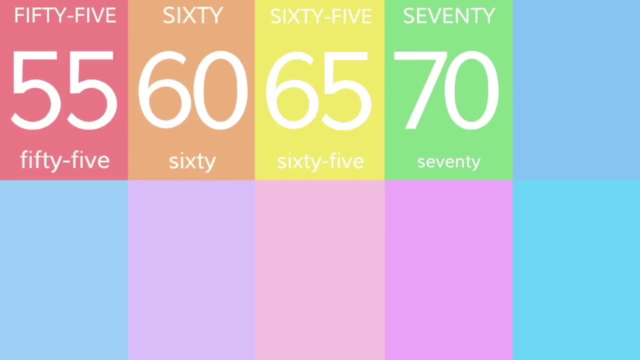 100.. 100.. Let's do it again. Let's do it again: 5,, 10,, 15,, 20,, 25,, 30,, 35,, 40,, 45,, 50,, 55,, 60,, 65,, 70,, 75,, 80,, 85,, 90,, 95.. 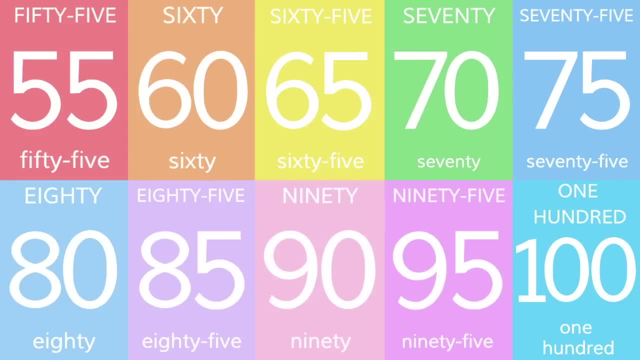 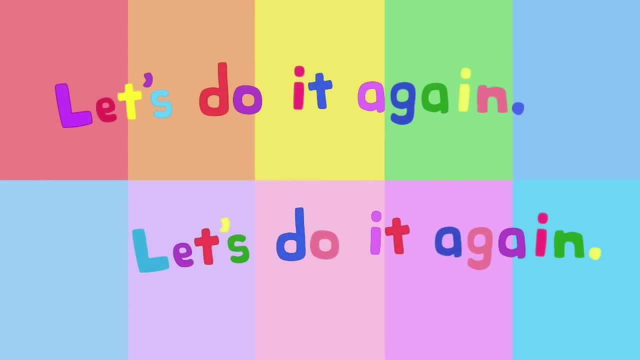 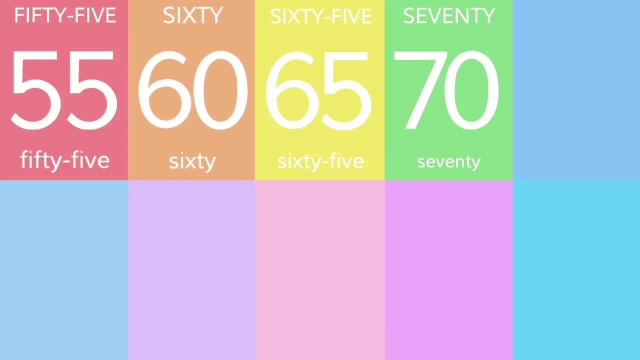 80, 95, 90,, 100.. 100.. Let's do it again. Let's do it again Again: 5, 10, 15,, 20,, 25,, 30,, 35,, 40, 45, 50,, 55,, 60, 65, 70, 75, 80, 85, 90, 95,, 100, 100. 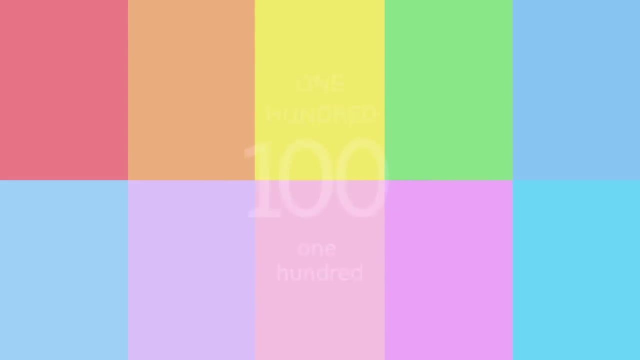 100.. Counting by fives, I know you can do it. Counting by fives, I know you can do it.